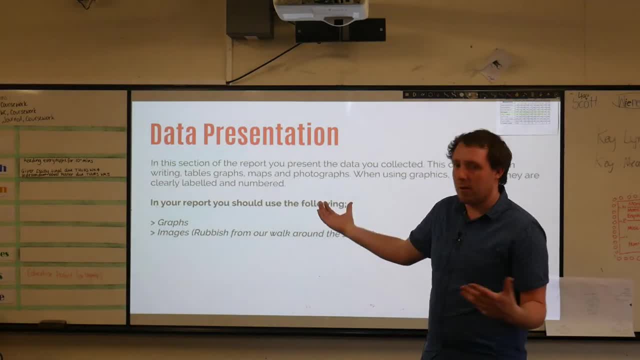 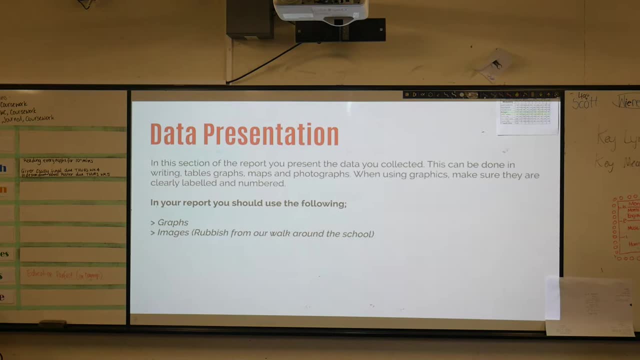 Because without that data, your field report really isn't a field report. Annalise, How do I present my data? Alright, So you can present your data in many ways, Alright. What we can do is: it's a little bit harder for you- Grass. 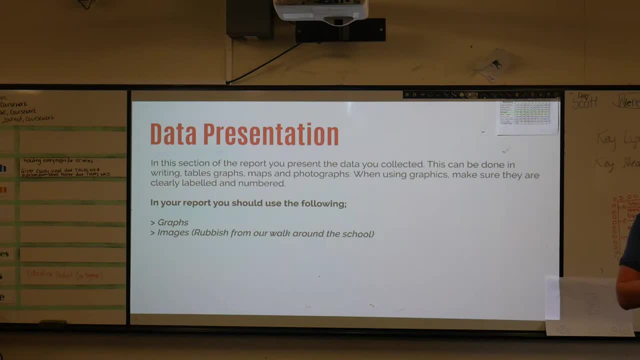 Okay, I will do one thing: The images that I've taken off the rubbish- okay, in bags. that is one form of data, So you will include those in your report, Alright, And you just say you can include a little caption. 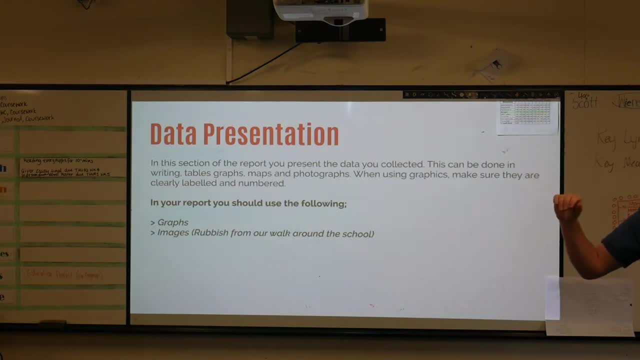 saying this is image collected from a field work session on Wednesday, the whatever of whatever 2019.. Alright, You will have a map, the map that you guys have done on that Thursday lesson last week. this time last week. 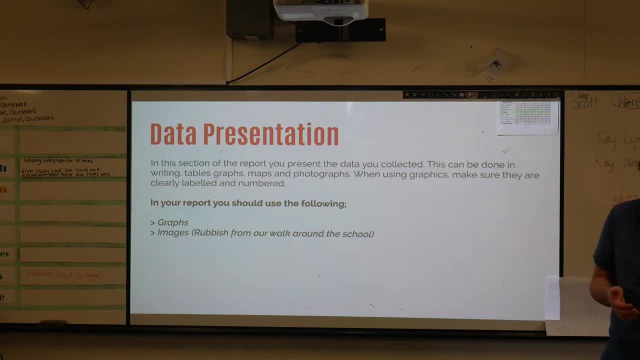 Those will also be put into you So I can get them from you. You can take a photo of them of your phone, put it onto your Word doc. You can bring them to me. I can scan them. It's entirely up to you. 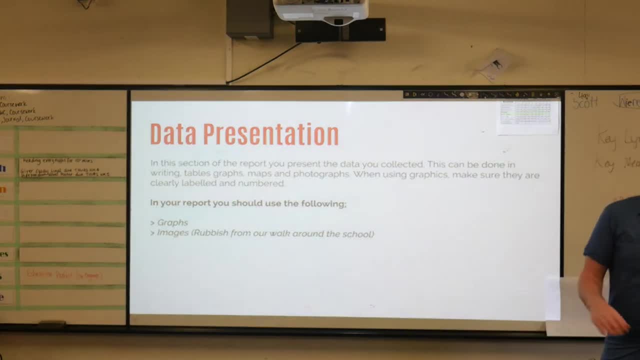 Alright, If you haven't done a really great job- bang up job on those maps last Thursday because some of you didn't, because we're just tired- then you're going to need to do those again. Alright, Your last one. 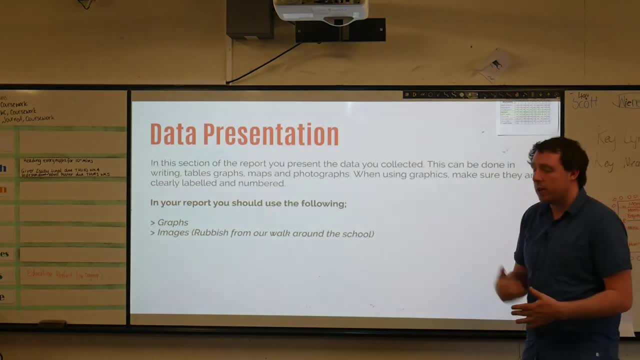 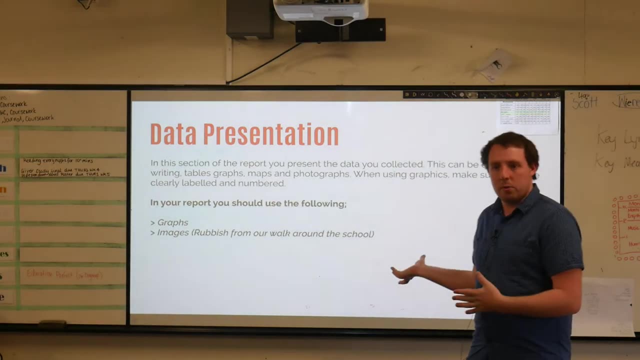 well, that's up to you. So, people who did surveys: okay, put them into graphs. Okay, Put that data that you got. put it to a graph. Okay, Images- well, same deal, You can put them into images. 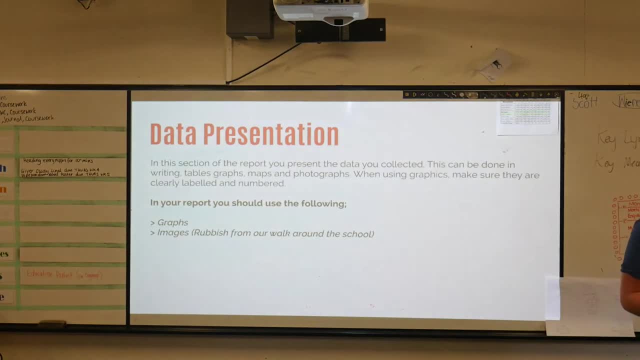 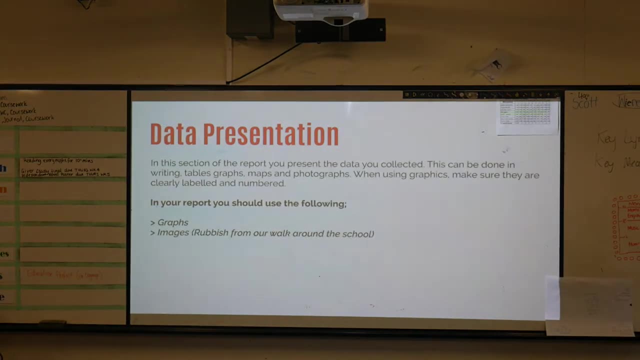 Okay, Outlining what they are and what they mean. If you've got a lot of qualitative research, like, or data- sorry, like your interviews, you can just put stuff into tables, Alright, And outline key, I guess key. 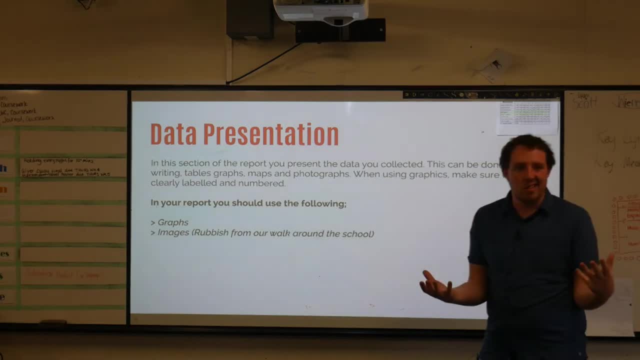 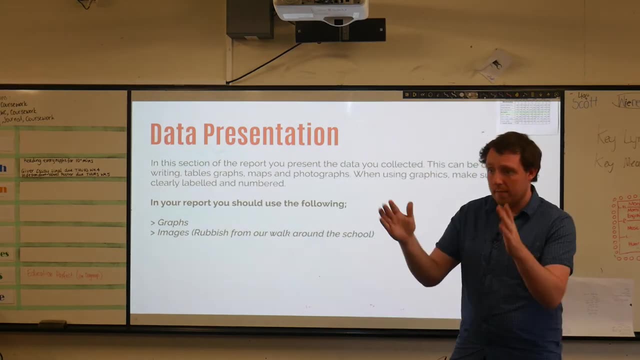 what's the word I'm trying to think of, Like key sentences, key things that we've- both Will and I- have said. Alright, Same applies, though, as well for your surveys: Any key responses that you got, you can put them in a table as well. 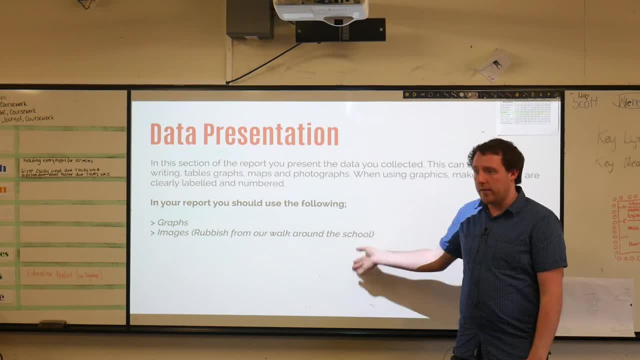 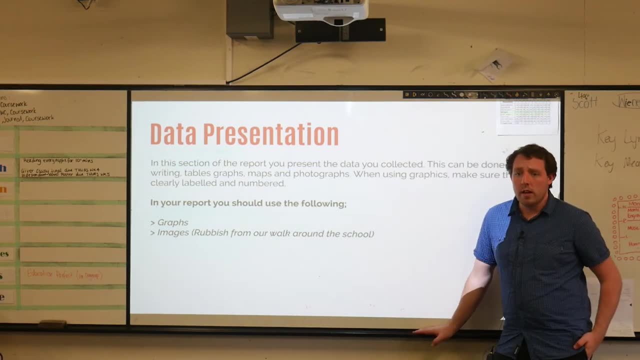 It is really important that your data is set up appropriately: easy to read, easy to understand. Alright, Yeah, you hand up Liv. Yeah, so, even if I started with just a graph, yeah, yeah, sure, sure. 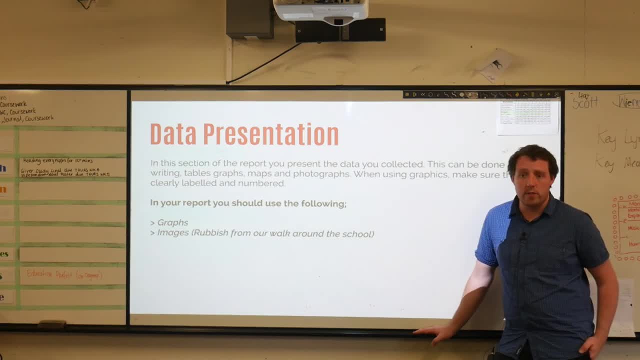 You could, yeah, yeah, there's heaps of things you can do, and we can have a chat about that as well. Alright, Alright.